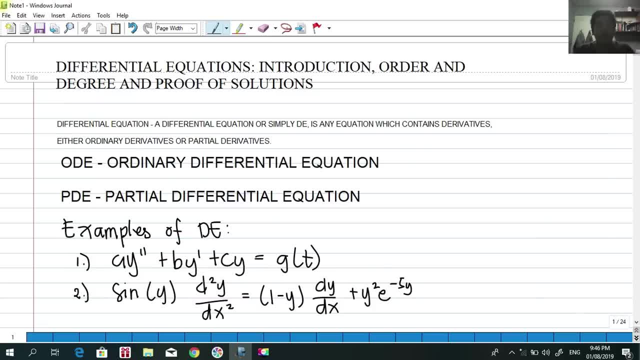 Basically, this is a video of an introduction, all about differential equation. So let's get started. First we need to define what is a differential equation. A differential equation, or simply denoted as DE, that's right. DE is any equation which contains derivatives. So I suppose 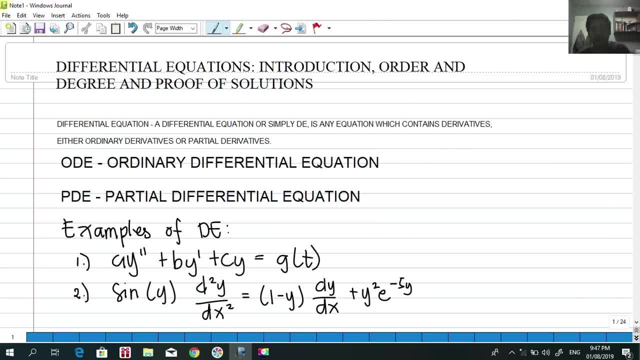 you are done already with your differential integral calculus because differential equations, you will be using your concepts again, recalling your concepts again in derivatives as well as the integral. okay, And is any equation which contains derivatives either ordinary derivatives or partial derivatives? So in differential equation we have what we call the ODE or the PDE. ODE stands for the ordinary. 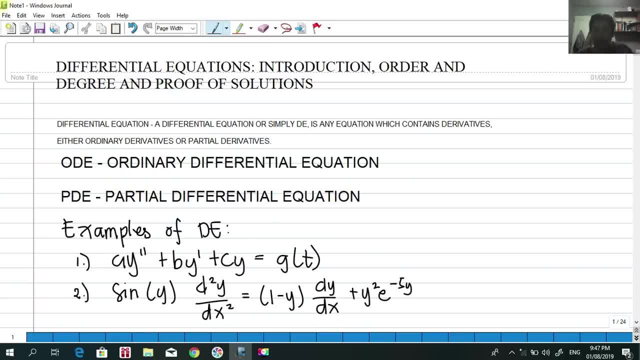 differential equations. These are the differential equation that has derivatives. okay, Not partial derivatives, but a pure derivative. Okay, For PDE. or partial differential equation. of course, from the word itself, it contains partial derivatives- Okay. Differential equation is actually a very broad topic, and here I have examples of differential. 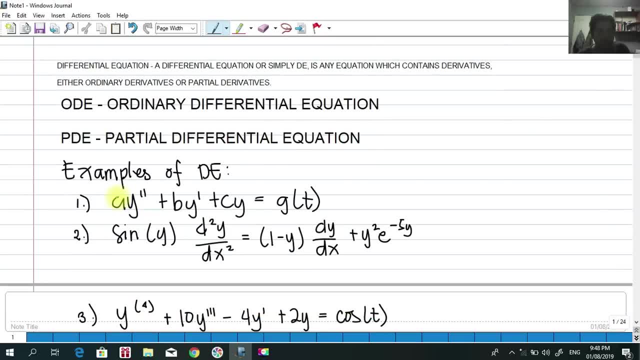 equations in here. So we have here this first equation, A multiplied by Y double prime, which denotes that Y double prime- oops, Y double prime- is actually the second derivative, So the second derivative of Y, maybe with respect to X, That is the second derivative. This is also equivalent to Y double prime, as we recall our concept in differential. 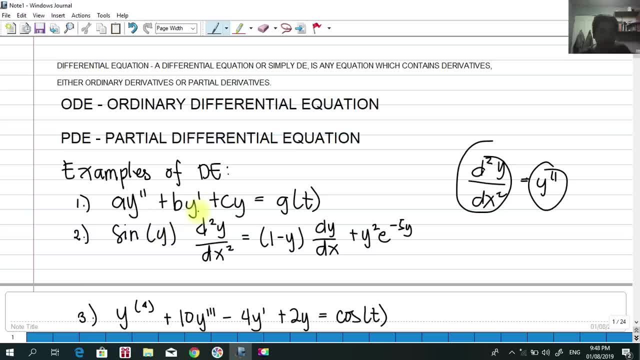 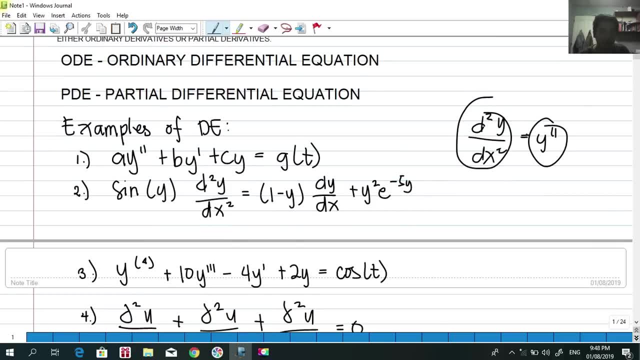 calculus. So ABC is any constant here in this case and that is equal to G of T. And for the second one we have some examples again of DE. Oh, by the way, the number one is actually this. number one equation of example of this is actually an ordinary differential equation. This is an ODE. 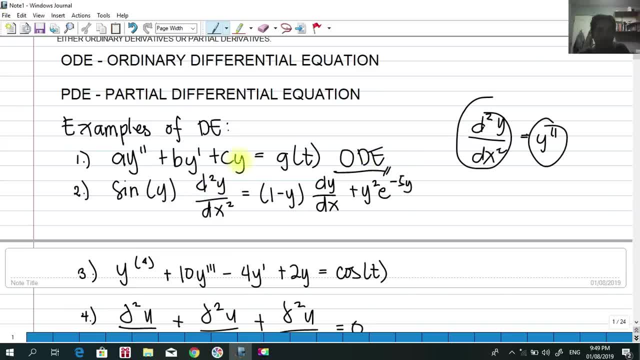 ä, Because it does not contain any partial derivatives in its equation. okay, So for number two, we have SIN X multiplied by the second derivative of Y with respect to X, And that is equivalent to one quantity, 1 minus 2.. 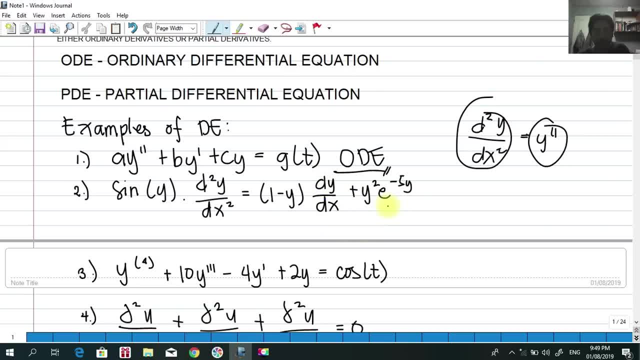 And the derivative of dy over dx plus y decreases squared times e raised to negative 5y. Now this is also an example of what. Is it an ordinary differential equation or a partial differential equation? Well, of course we don't see any. 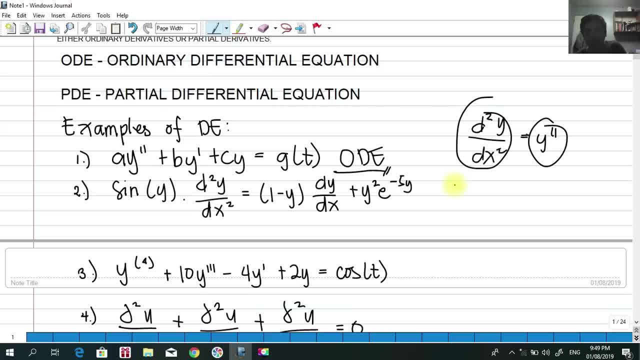 partial derivatives here in our equation, so we can conclude that this is an ordinary differential equation. okay, So it seems complicated at first, but as we go on in our lesson, you will actually would try to solve this kind of equation. We will be dealing a lot with this kind of equations. 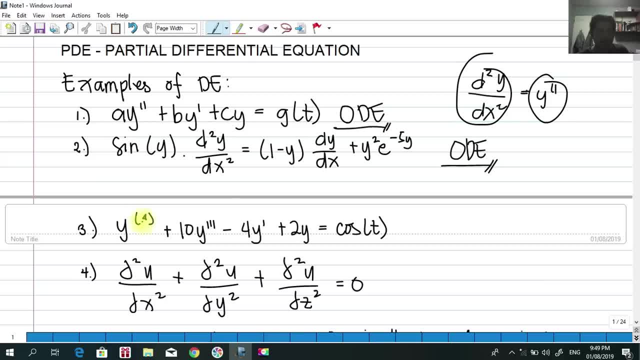 okay For number 3, that is, y raised to negative, y raised to 4.. Take note that this y raised to 4 with a parenthesis here, is not equivalent to simply y raised to 4.. y raised to the quantity of 4 here denotes that it is the fourth derivative. okay, Fourth derivative. 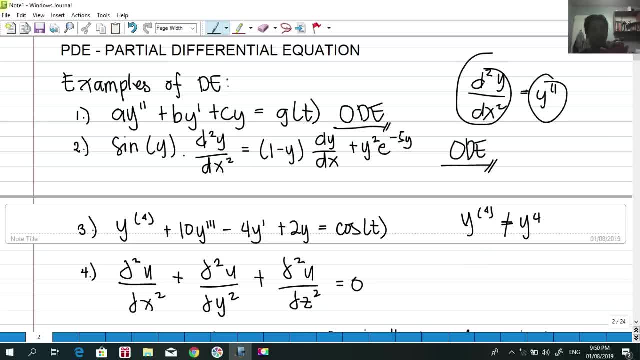 of y With respect to some certain variable. maybe it's x, okay. So fourth derivative of y plus 10, the third derivative of this y triple prime minus 4y prime, the first derivative plus 2y, is equal to the cosine of t And actually, if we're going to analyze this again, this is an. 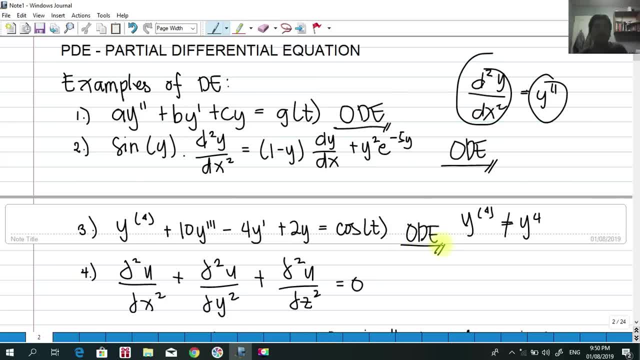 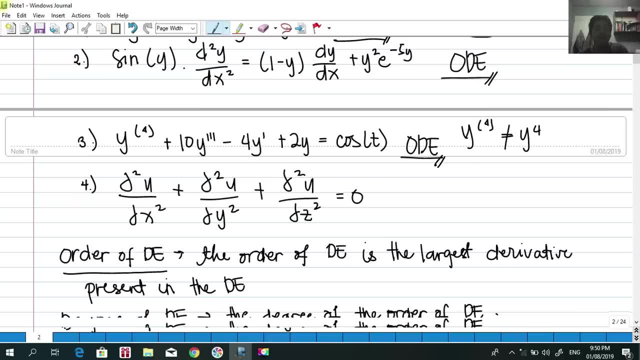 ordinary differential equation because it does not contain any partial derivatives in the equation. Okay, I hope you're getting what I'm trying to say here. okay, So for number 4, obviously this is a partial differential equation because it contains partial derivatives denoted by this symbol. okay, 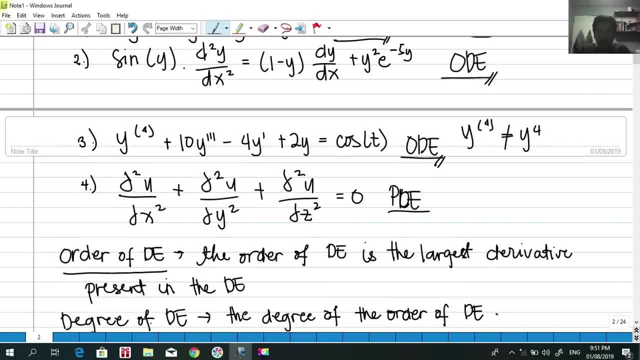 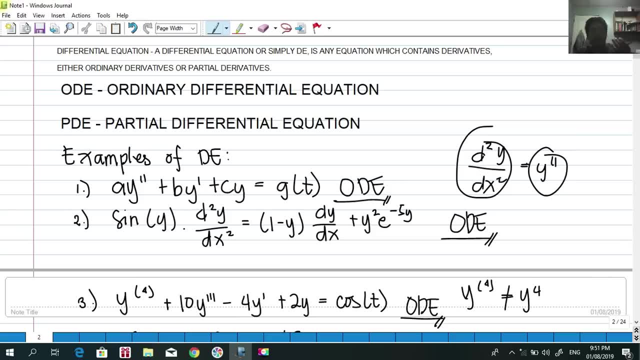 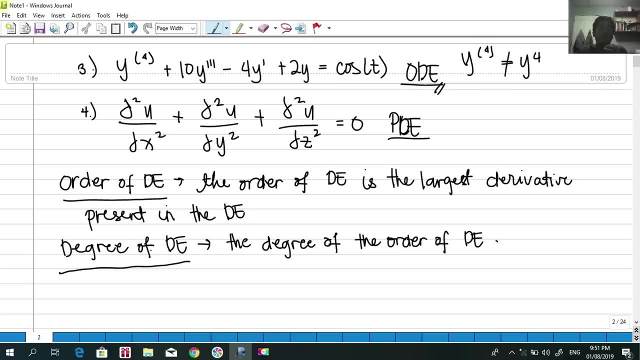 The partial derivatives. So that is an ODE and PDE. That is the two type of our differential equations. We have the ODE- ordinary differential equation and we have the partial differential equation. So we have what we call in order for us to fully understand first before we solve. 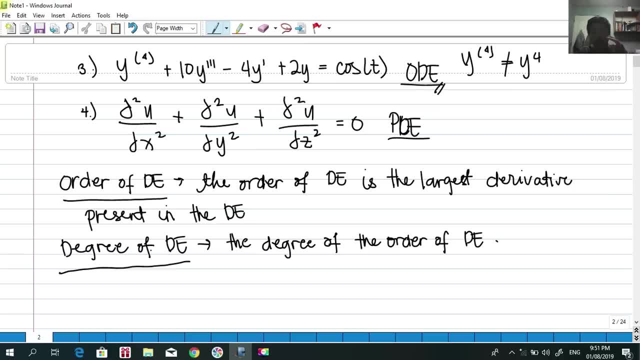 some DE. we need to understand a very important terms in DE, And that is what we call the order of the differential equation. and this order of the differential equation and the degree of differential equation. What are these two terms? So the order. when we talk about the order, 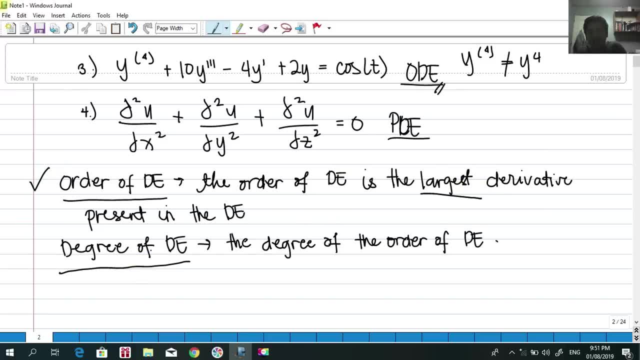 the order of the DE is the larger, The largest derivative present in the DE, free from square roots. okay, Free from square roots, free from the inside function of a transcendental function. Of course that is the order DE: the largest derivative, the highest derivative of the equation. okay, That's the order. How about? 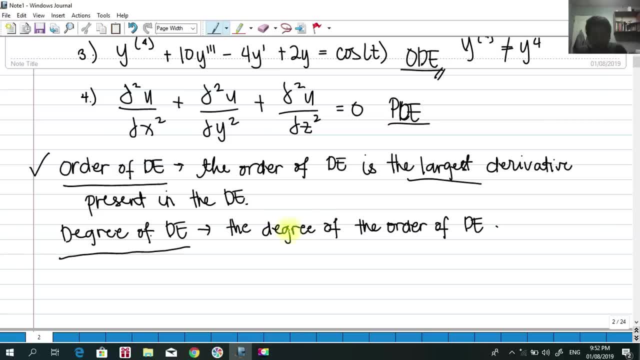 the degree. The degree is actually the degree of the DE, is the order of the DE. So the degree of the DE, okay, is defined by the order of the DE. So the degree of the DE is defined by the order of. 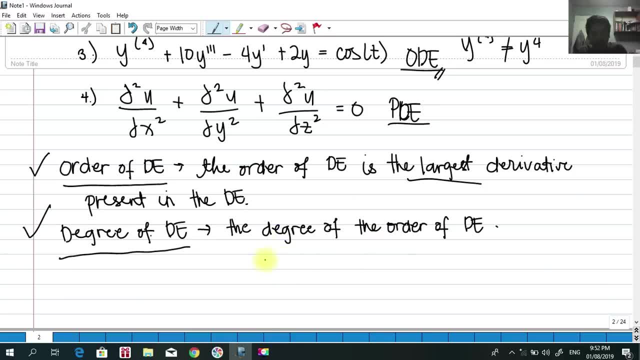 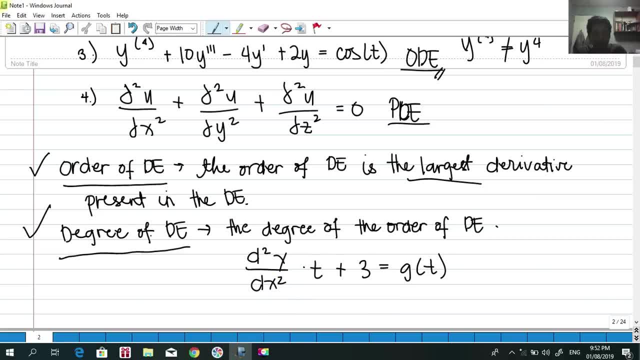 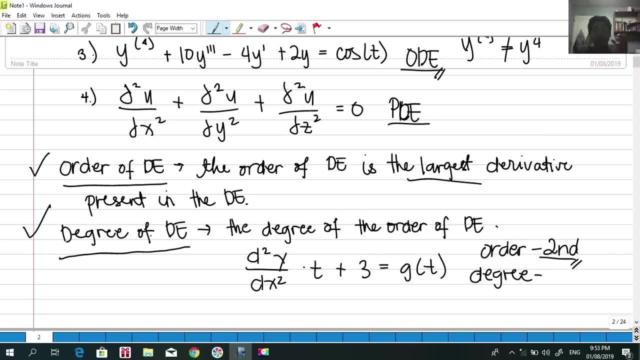 The degree of the DE is actually the degree to which the order of the DE is raised. So if this is our order, second order, what is the exponent of this? Well, of course that is one. So our degree is first degree. 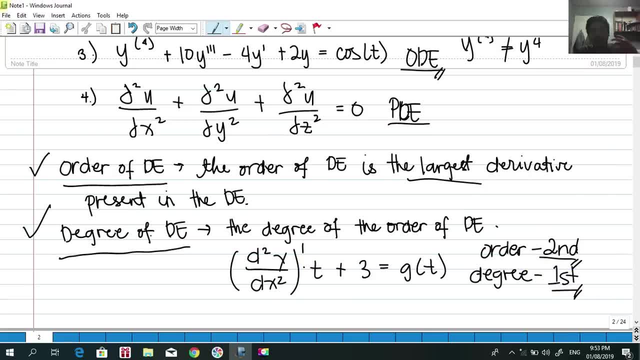 okay, i hope you get the the definition of the order of the d in the degree of the d. so we will try to solve, or we will try to practice by finding out what is the order in the degree of a certain d. okay, i have so many examples here and let's try to determine what is the order and the degree. 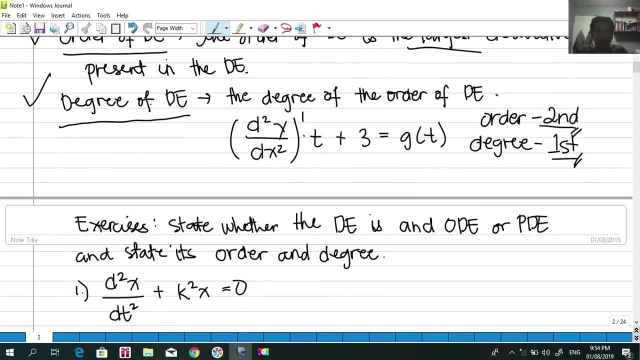 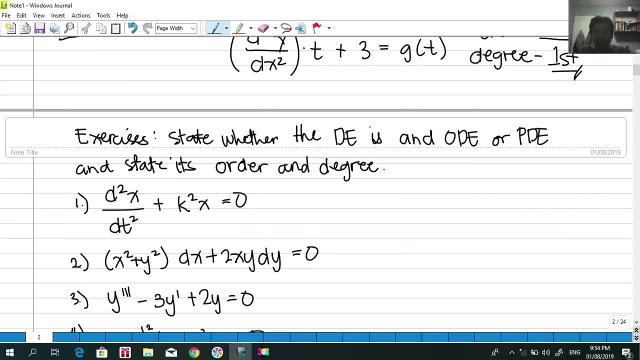 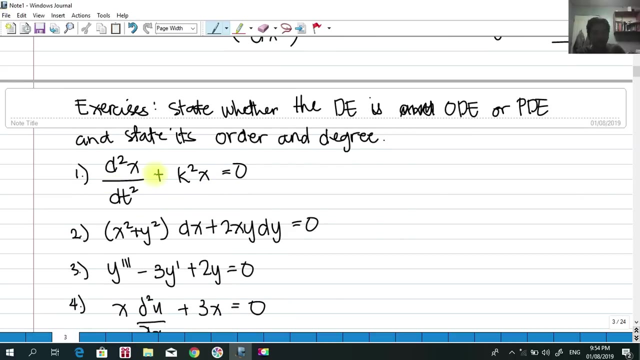 of the differential equation. so, for number one, here are our exercises and this is the. the instructions state whether the d is, of course, is ode or pde, and state its order and, at the same time, the degree. so for number one, we have this differential equation. okay. so, since this, 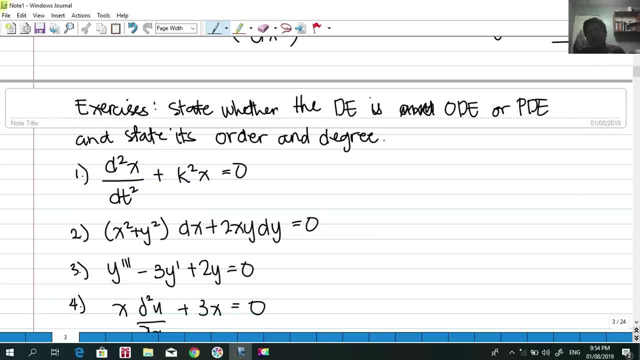 differential equation does not contain any partial derivatives, then definitely. our answer is: this is an ode, ordinary differential equation. well, how about the order in the degree? first you need to determine the order. so the order of this differential equation, since this is second derivative, the order is actually what order of two or second order? okay, and its degree is. 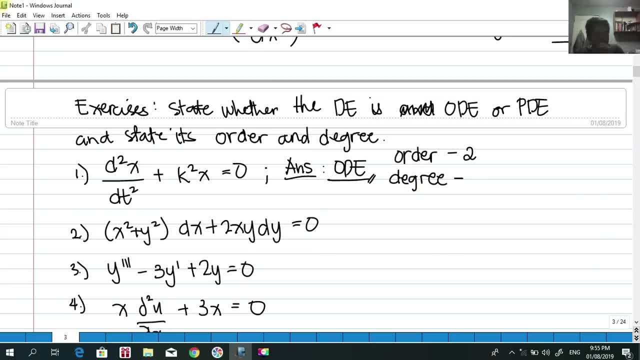 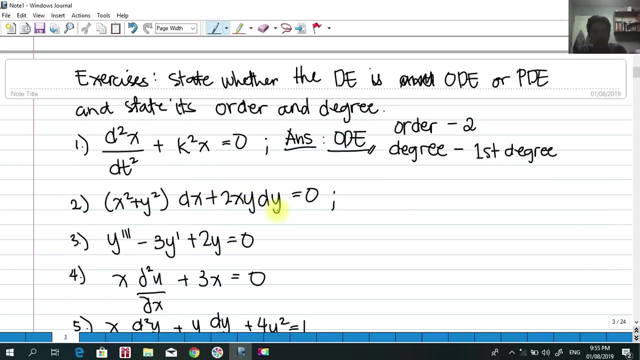 the exponent of the order. so the exponent here, in this case this is one or first degree. so in other words, this differential equation is: uh, has an order of two in a degree of a first degree. okay, so for number two, we have here this differential equation. so we have this x squared plus y squared, dx plus 2x d, what is equals to zero. 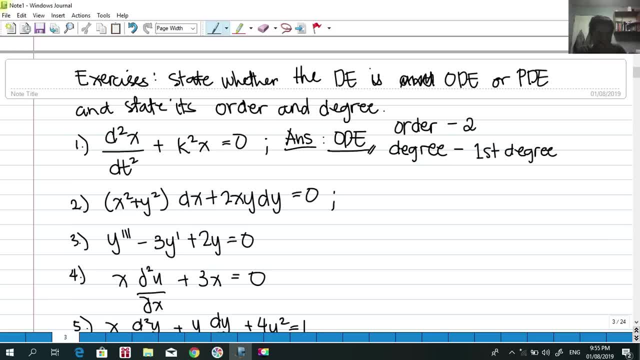 okay, how do we know the order in the degree? first of all, uh, we need to multiply the whole equation. for us to see this, we need to multiply the whole equation by 1 over dx so that we can determine the dy over dx. if we do that, 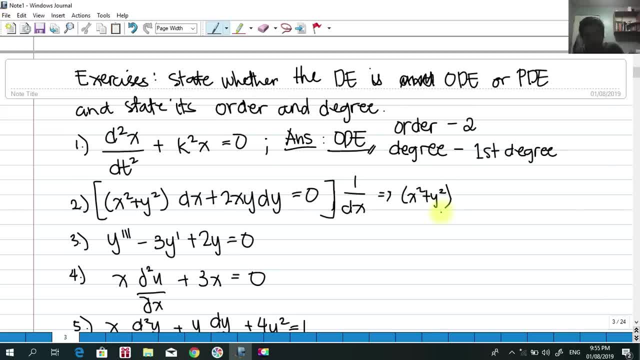 what will happen? x squared plus y squared, dx will cancel plus 2xy. so we have now the dy. the dy here over dx is equals to zero, and then we're going to determine what is now the order or degree of this. first of all, this is an ode, because it does not contain any partial 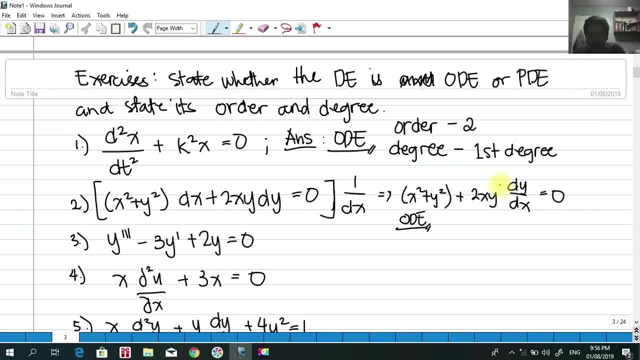 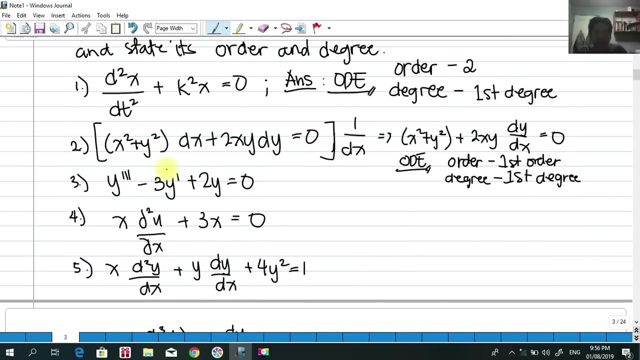 derivatives in it and uh, we have here a derivative. our order should be first order, okay, or order of 1, and our degree is again the exponent of our order and that is also first degree. so our answer is o d, first order, first degree, order of one, first degree, okay. so for number three we have here, it's very obvious. so this is an ode. 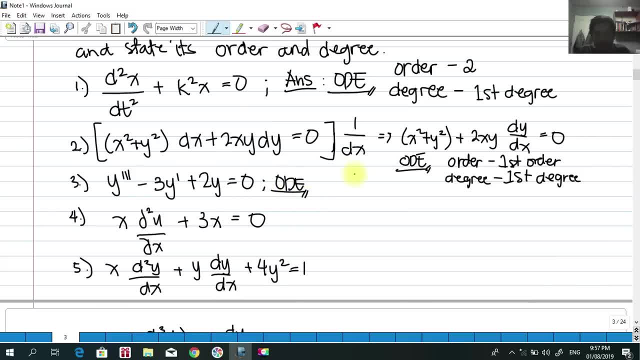 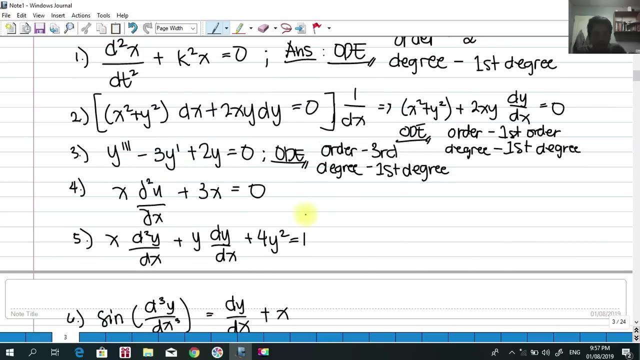 of course. what is its order again from this equation? what is the order of this equation that's a order three or third order, okay, and the degree is actually what? first degree, okay. and of course, for number four, this is a partial differential equation because it's as 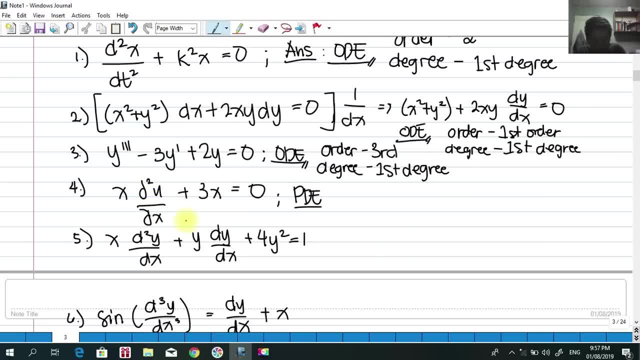 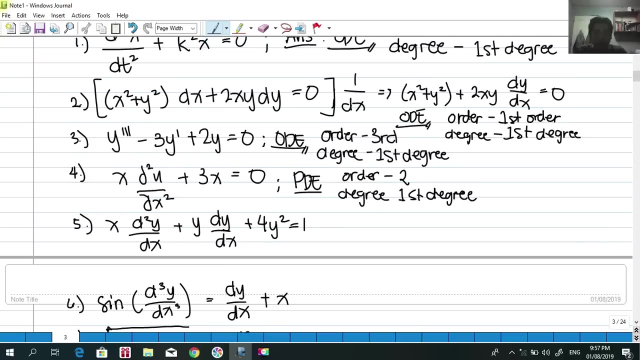 a partial derivative here and of course, this has a two here, so its order is actually what? yes, that's a order of two and our degree is what? first degree: okay, i hope you can actually uh follow my uh lesson here. okay, i hope you are not lost. okay, it's okay, i know it's easy. 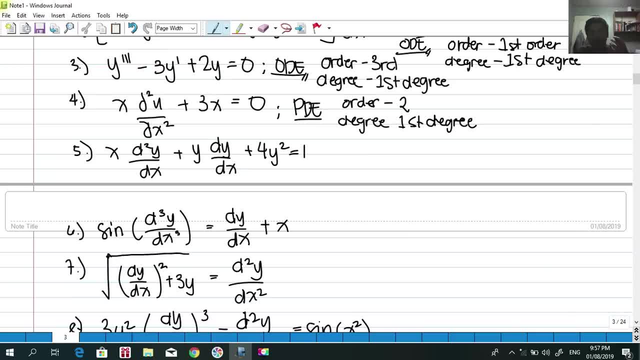 we're going to- uh, we're going to- tackle a little bit hard topic when we go on solutions of de. okay, for number five, we have- of course this is an ode- ordinary differential equation, because, again, it does not have any partial derivative. it doesn't contain any partial derivatives in. 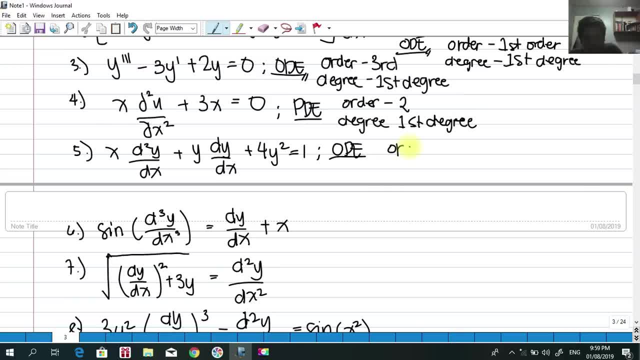 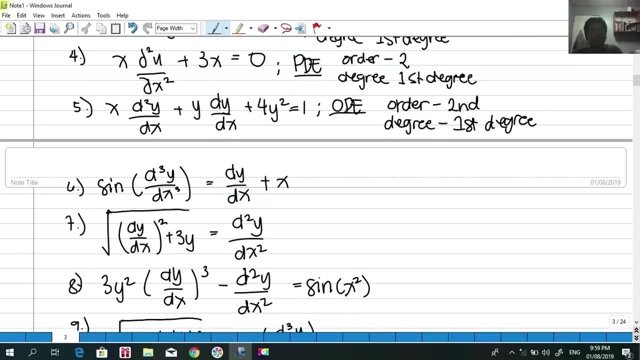 its equation. so, and what is the order? okay, that's the order. that is the second order, differential equation. and what's the degree? well, of course, the degree. the degree is first degree. okay for number six, for number six. we need to be careful in determining the order and the degree. 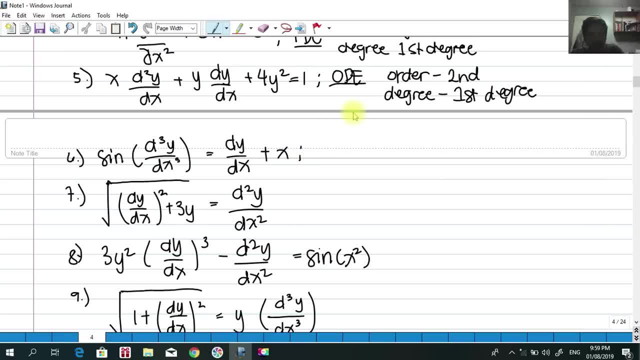 of this differential equation. okay, what is this? this is an ordinary differential equation. okay, now my question is: what is the order? think about it. you might say that the order is a third order or third degree order of order of three, but definitely, as i've said a while ago, that the order depends on the highest derivative. 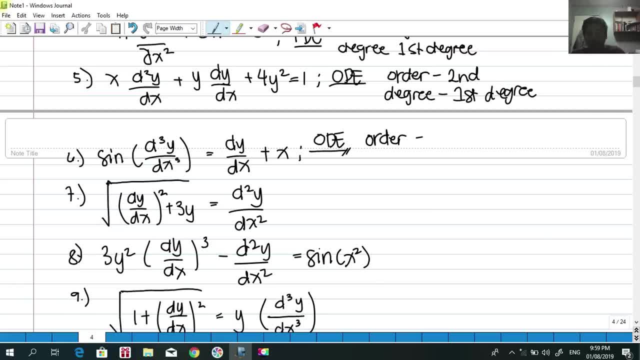 not inside a transcendental function but existing as an independent differential or derivative. so, in this case, sign off the third derivative of y with respect to x. no, this is not the order of these. The order of this differential equation is not 3, Because the derivative is actually inside the transcendental function. 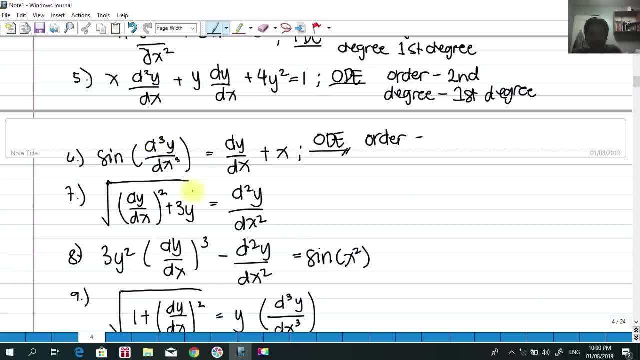 When this happens, this is not counted as the order of the DE, But rather, if we look at this on the right side of the equation, We have dy over dx here And this exists as independent, free from radical, And not inside the transcendental function. 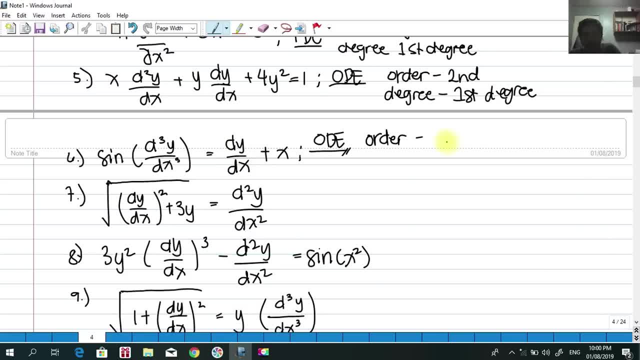 So, therefore, we can say that the order of this differential equation is a order of 1 And its degree actually is first degree. Please remember that We cannot actually choose 3 as our order. Why? Because, again, the derivative is inside a transcendental function. 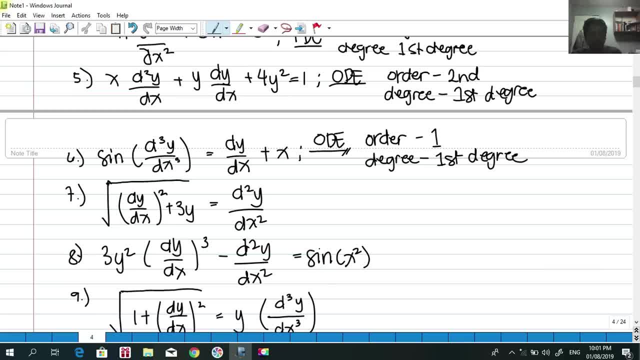 Okay, That is not our degree, But rather if we choose, If we choose the derivative existing as its own derivative, As an independent, free from radicals, And not inside the transcendental function. That's the order of our degree. Okay, For number 7, actually. 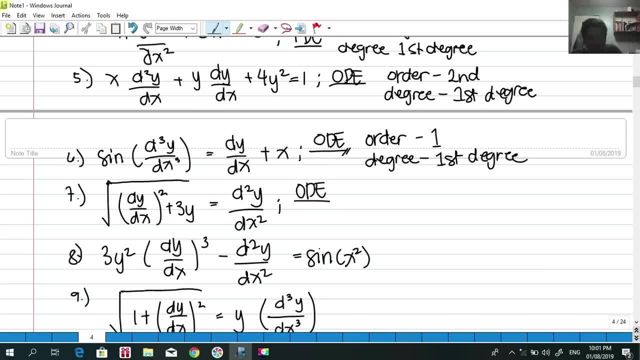 This is an ODE. Again, Why? Because it does not have any partial derivatives inside the equation. And again, in order for us to determine The degree and order of this differential equation, We need to somehow modify the equation Or simplify the equation If I'm going to square both sides of the equation. 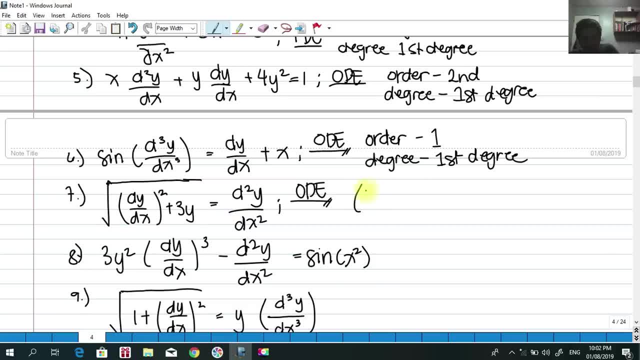 We shall eliminate the square root And this will be our answer. dy dx squared Plus 3y Is equals to The second derivative of y With respect to x squared. Now, Okay, You can now determine the order and degree Of this differential equation By actually eliminating the radical. 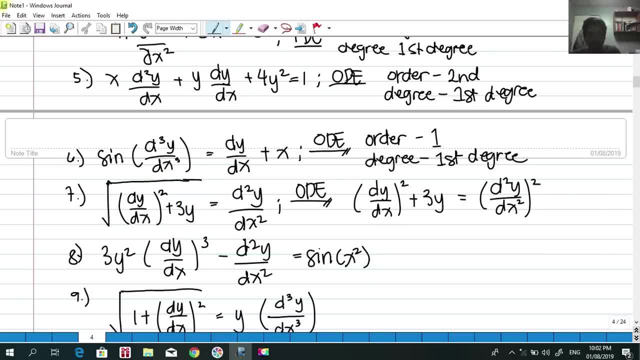 That is the rule. If you see a radical, Eliminate first the radical And then Find the order and the degree. So We're going to analyze this. Our order now will be: what Order is now The highest derivative? Of course We have a second order, Order of 2. 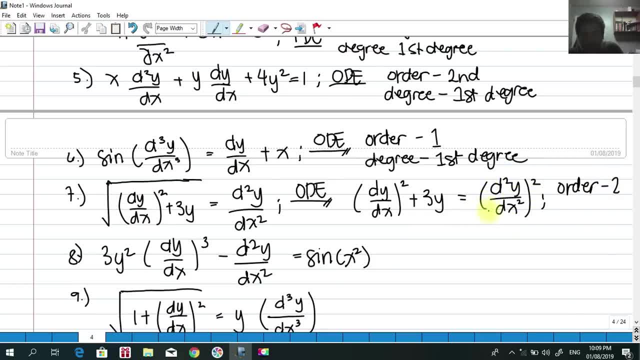 Because of this. Okay, This is a second derivative, While this one is a first derivative. Now, what will be our degree? Of course, As I've said, The degree is actually The exponent of the derivative of y, The exponent of the derivative of y, The exponent of the derivative of y. 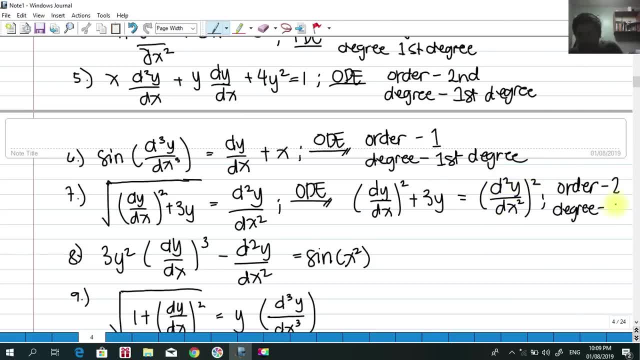 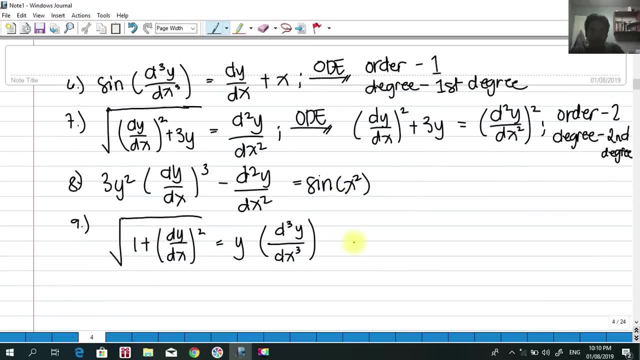 Of the order. So if this is our order, What's the exponent? That's a second degree Differential equation. Okay, moving forward. So we have this equation again, This is an ODE Because, again, it does not have any partial derivatives Inside the equation And, of course, There's no problem in determining the order. 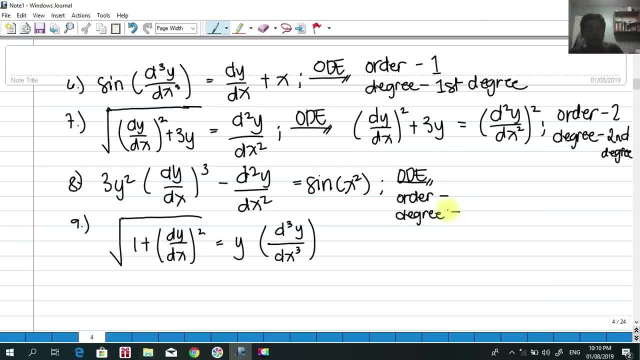 Or the degree here, Because we don't have any square roots. Because we don't have any square roots. Okay, Of course, If we're going to determine What's the order and the degree, The order actually is what The order is. second order- Order of 2. 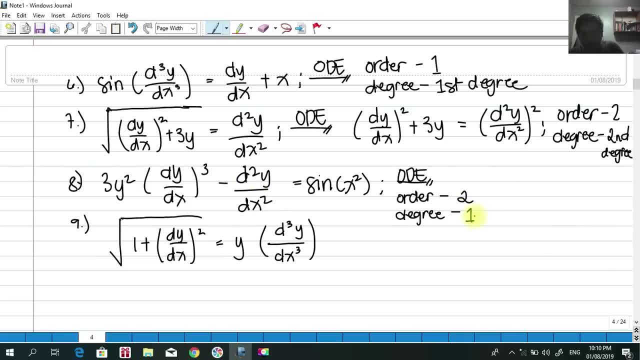 And how about its degree? First degree, Okay, Don't be tempted To actually think That this is the degree Okay, Because actually the degree is The exponent, again, Of the order, Of the derivative Or the differential equation, And in this case, This is our order. Its exponent is actually 1. 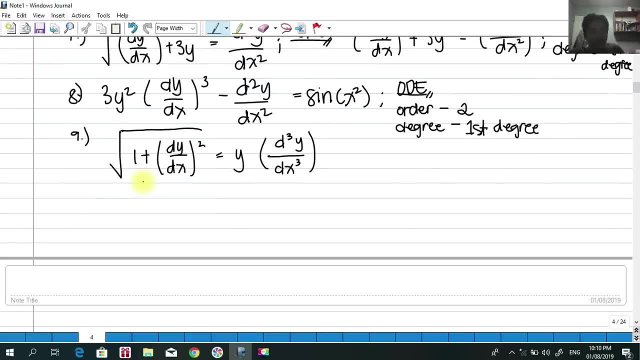 So we got this answer. And for number 9, Lastly, we have This expression: We have to square first Both sides of the equation So that we have 1 plus dy Over. dx squared Is equals to y squared. Third derivative of y With respect to x Squared. 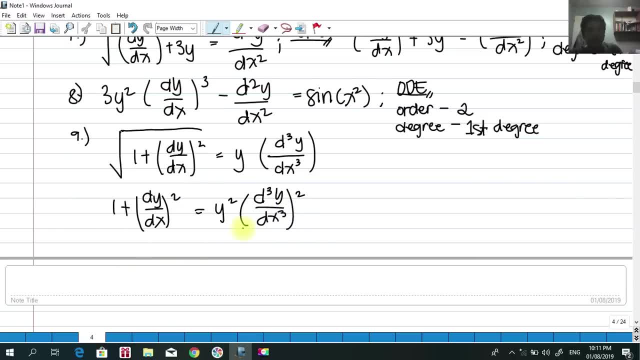 Okay, If we reduce this Differential equation Into this, If we eliminate the radical, Then we can say, Now that we Are safe, now To find the order And the dE, Or the degree Of this differential equation. By the way, This is an Ordinary differential equation. Okay, So order. 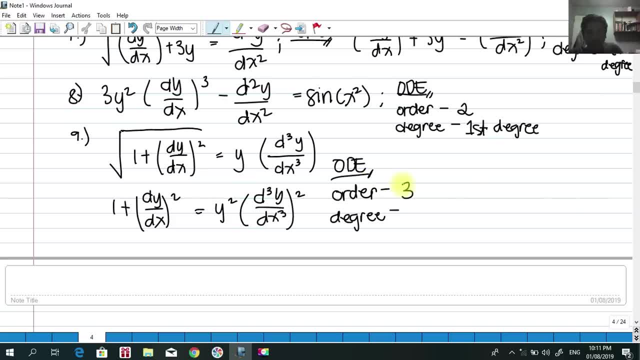 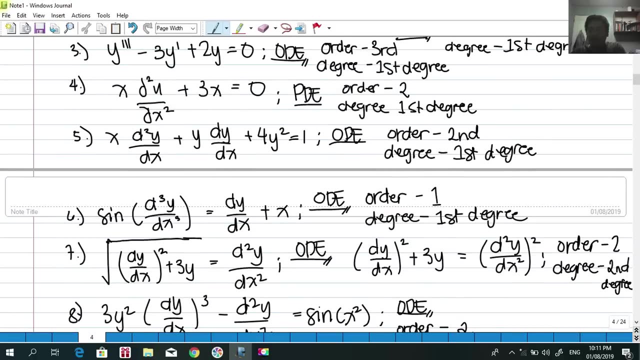 What is the order? That is Order of 3 Because of this Third derivative, And the degree Is actually Second degree. Okay, That is the order And the degree Of our Differential equation. Now Let us try To move on now In solving Or showing A proof Of solution. 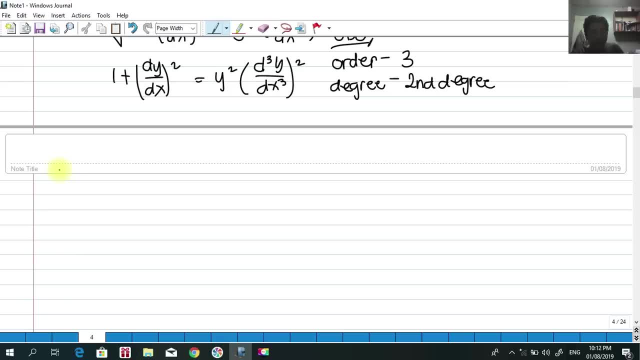 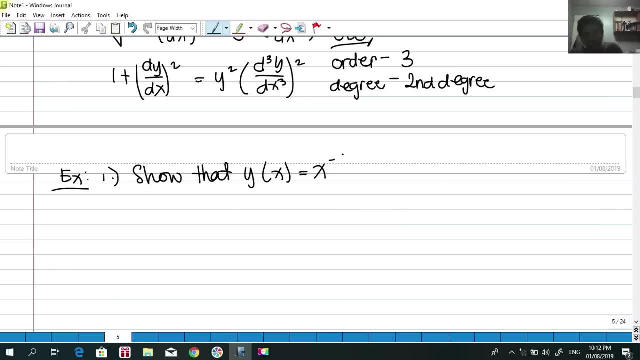 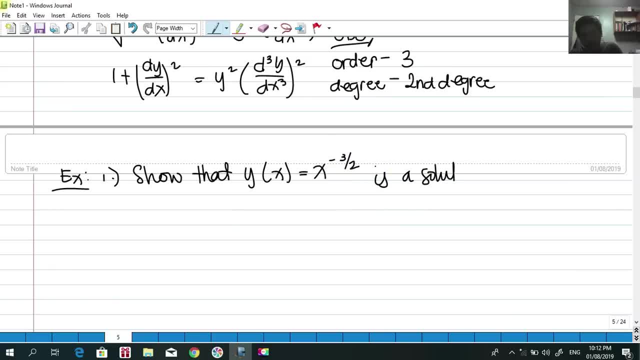 3, 3 Is a solution. 2, The d 4 X 4, 4 Y, Y Y, Double Y Plus 12 X Y Y, Prime Plus 3 Y Is equal to 0, 4 X Greater than 0, As I have said A while ago. 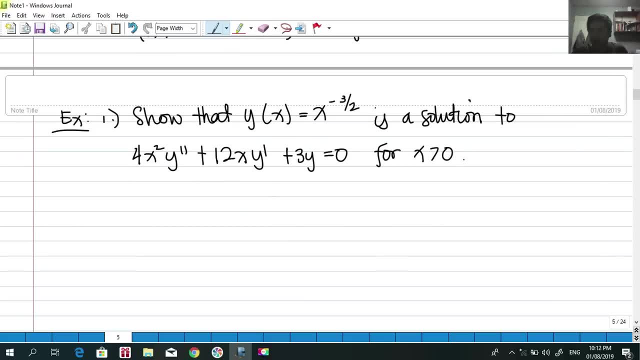 In Studying differential Equation You will be calling your basic differential calculus and any integral calculus. for the latter part of our discussion, and in here, what are we going to do in this differential equation is to prove that this y of x, x is equals to a. y of x equals to x raised to negative three halves is a solution. 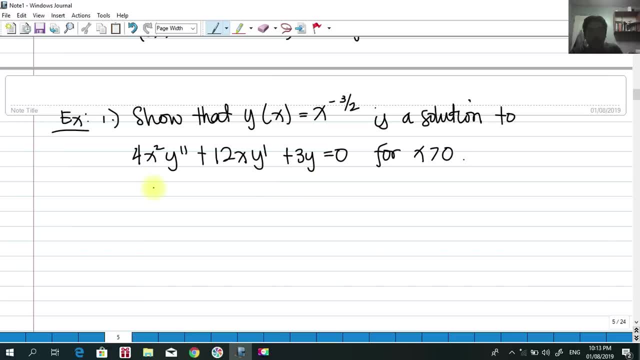 for this differential equation. what do we mean by that? if we are going to perform, uh, if we're going to substitute this value into this differential equation, it should result to a zero. remember, in your algebra, if a certain value of x is a solution to that polynomial. 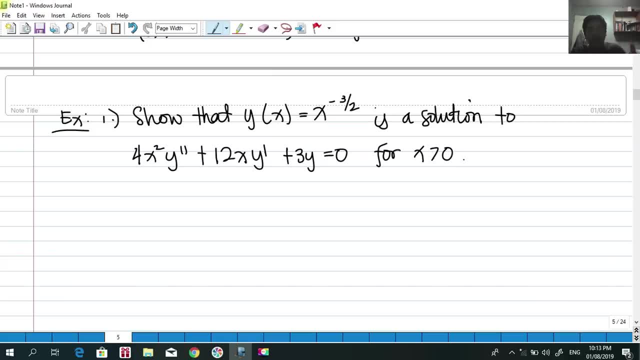 given the, the answer should be zero. it should satisfy the equation here. it's the same solution. when we talk about solution, it is actually solution. when we talk about solution, it is actually solution. when we talk about solution, it is actually, let's say, in a polynomial, that is a root that would equal to zero. 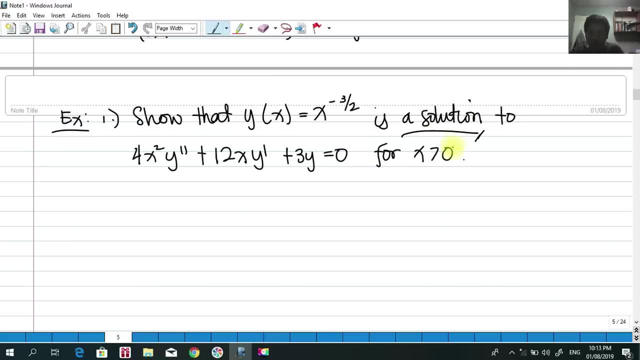 but in this differential equation it is also called a solution. but the difference is that this differential equation actually involves derivatives. so what are we going to do? first, the solution in our solution. okay, since we know y of x, or simply y, and that is equal to x raised to negative three halves, we know that we need to get the first. 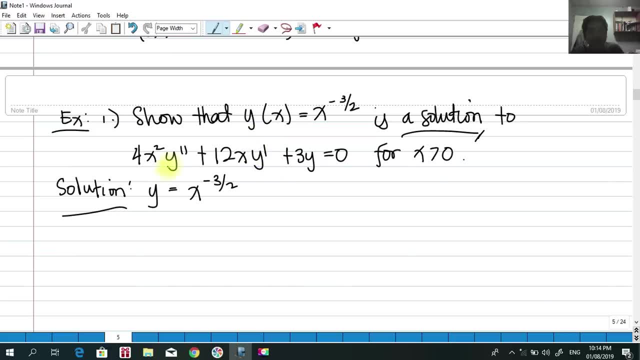 derivative, because this is y prime. this is first derivative and the second derivative of this y, if we are going to find the solution for this differential equation. so again, if we get the first derivative, we have negative three halves x, negative three halves raised to negative three minus one, and that is negative three halves x raised to negative five halves. that is our first. 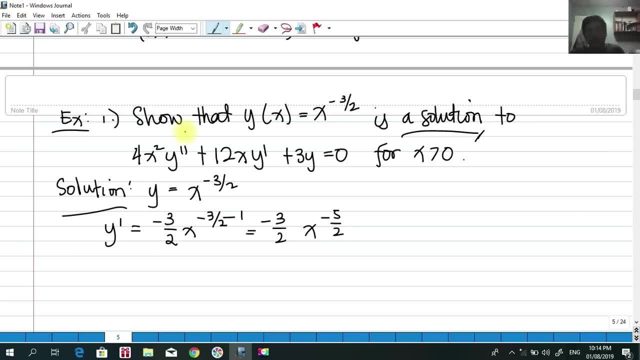 derivative and take note that in our differential equation we should also get the second derivative, y, double prime. so this is the first derivative. what will happen by power rule? we have negative three halves multiplied by negative five halves, x raised to negative five halves minus one, and we are going. 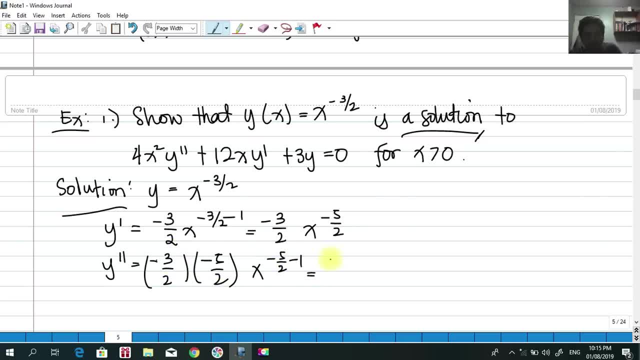 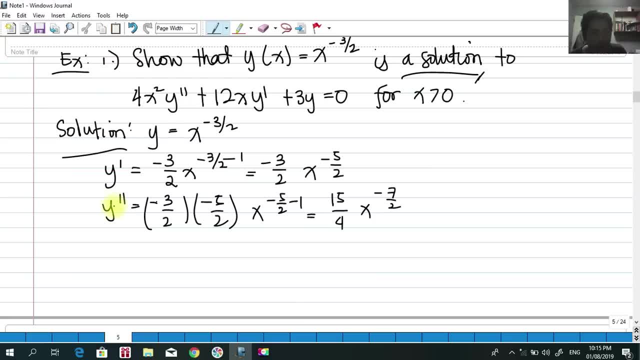 going to plug in this y prime and y double prime in our equation, in our differential equation. so what will happen is this: we have 4 x squared, y double prime is 15 over 4 x, raised to negative seven halves, okay, plus 12 x times. 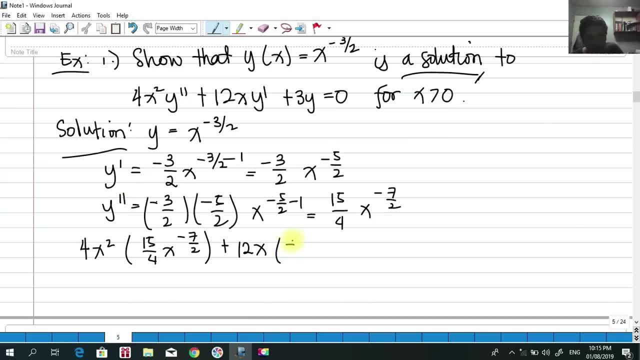 y prime, which is our y prime, is negative three halves. x raised to negative five halves- okay, plus 3 multiplied by y, which is this x raised to negative three halves, and that is equal to zero. so simplifying this: we have force will cancel. okay, so we have 12 over. 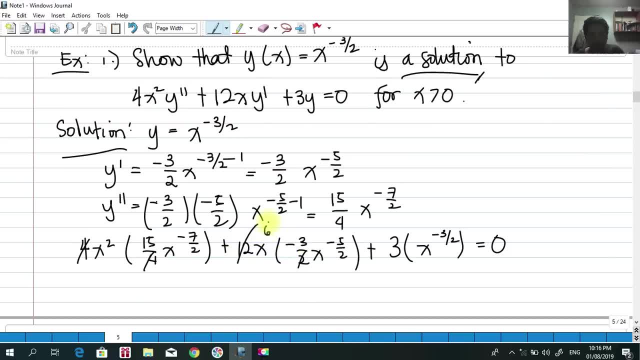 2, that is 6 here, 6 in here. then, yeah, we need to simplify this. so what will happen here is that 15 x squared multiplied by x, raised to negative, seven halves. okay, plus, or rather that's minus, because 6 times negative, 3 is negative. 18 x squared multiplied by x, raised to negative seven halves. 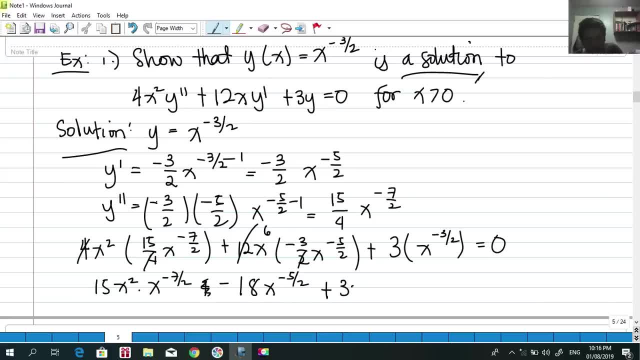 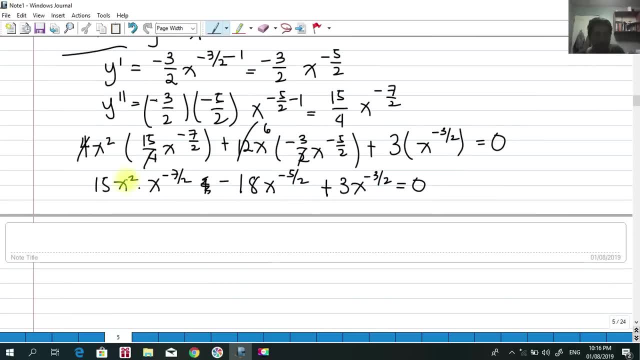 is equal to zero. on the 15 x squared x is equal to: oh, three plus half of x is x is equal to zero. okay, unfortunately, at the point where i'm using an element of x for x raised to negative 3. so this is x to x half and thats x to x raised to 5 and that, added up, is in the wrong way. so 35 l and 2x to x raised to five half, plus x to x, xh is equal to zero. this equals zero. now we're going to simplify this. 15 x squared x need to what we need it to. 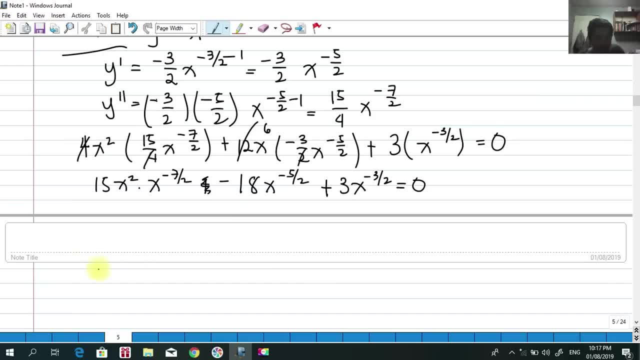 We need to actually does this to, so what will happen is 15x 2 minus 7 over 2. then we need to actually uh add this to, so what will happen is 15x 2 minus 7.. okay, we add y, we add here, we add the exponent: uh. there's no addition here because of the negative. 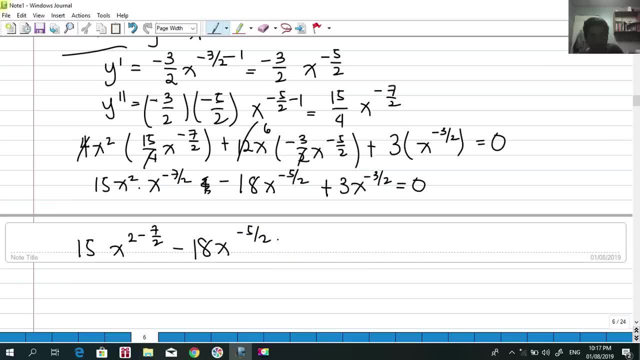 so we have negative 18x raised to negative 5 halves, plus 3x raised to negative 3 halves is equals to 0 and performing this we have 15, 2 times 2, 4, 4 minus 3. that is x raised to negative 3 halves. 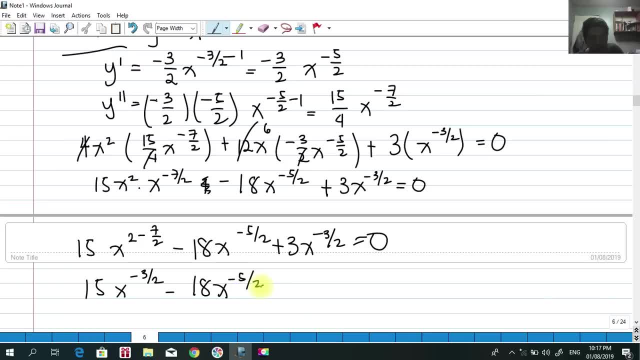 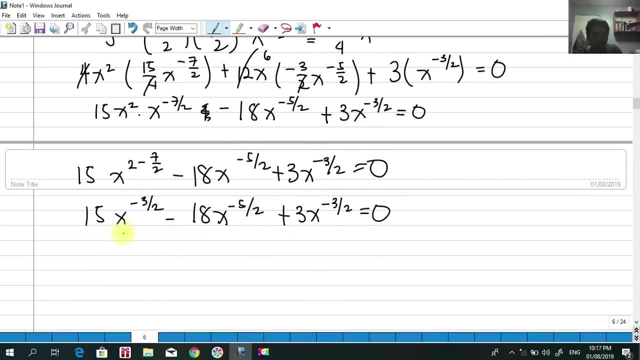 minus 18x raised to negative 5 halves, plus 3x raised to negative 3 halves. now, if we're going to combine like terms, okay, 15x raised to negative 3 halves plus 3x raised to negative 3 halves, minus 18x raised to 5 half. so what do we have here? that is equivalent to 0. 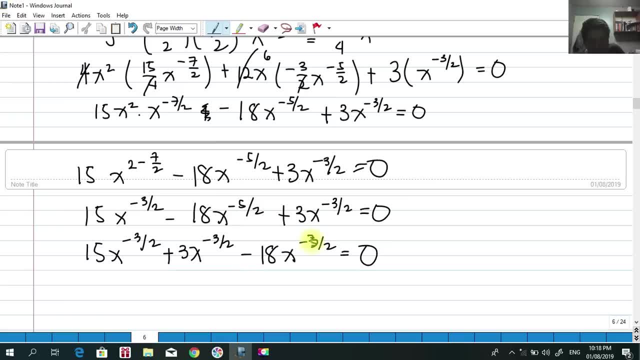 0. of course this is not 5 halves, but rather this is 3 halves. so if we're going to simplify this, 8x raised to 3 halves- 18x- i mean 15 plus 3 minus 18x- raised to negative 3 halves- is equals to 0. 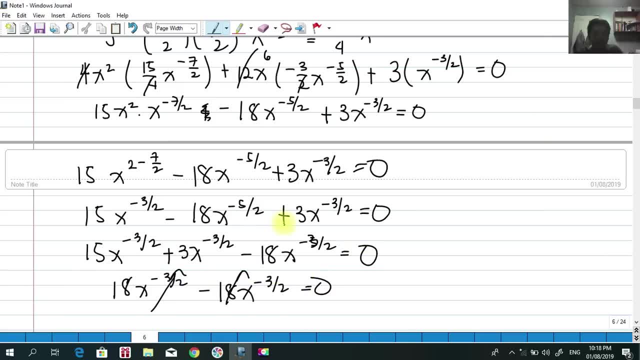 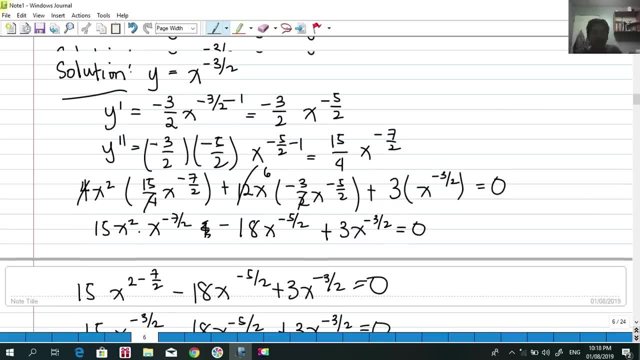 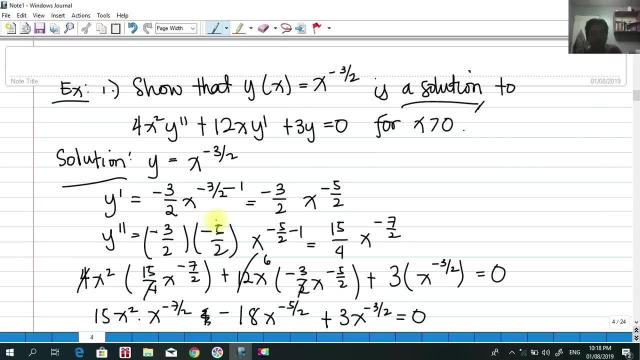 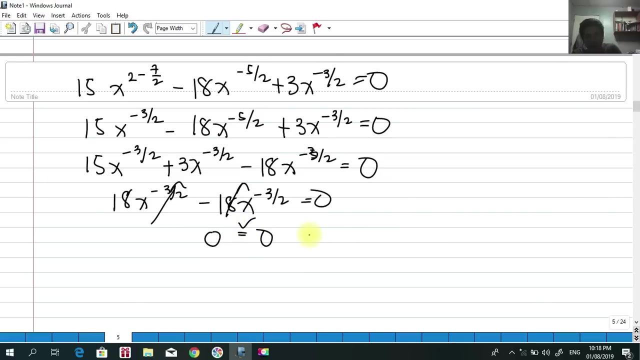 and definitely these two will cancel. so we have: 0 is equals to 0 and that only proves that this given function of y of x is equals to x raised to negative 3 halves is a solution for our de given de here. why? because it satisfied the equation 0 is equals to 0. so 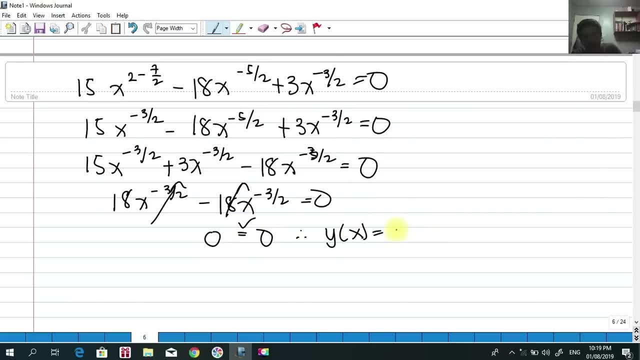 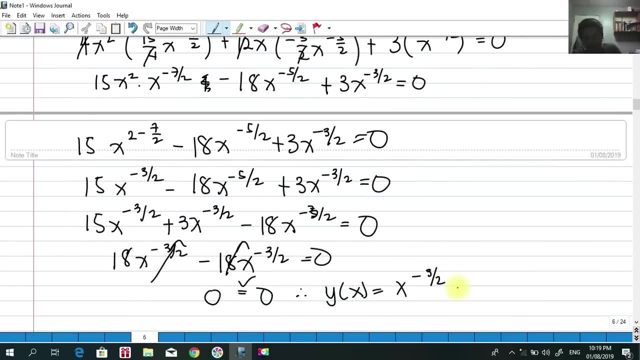 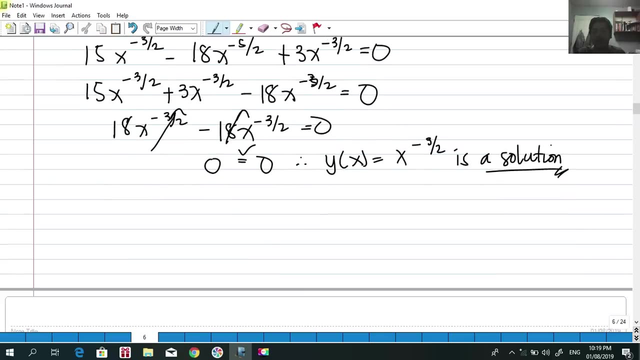 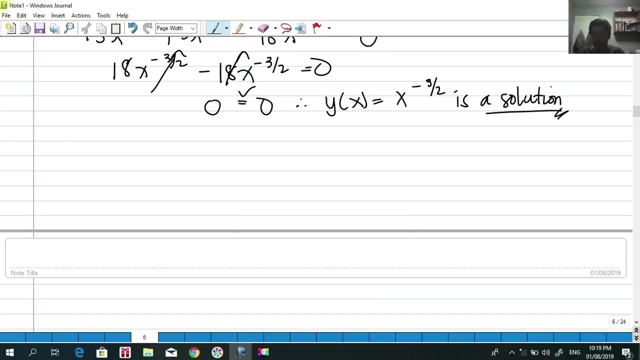 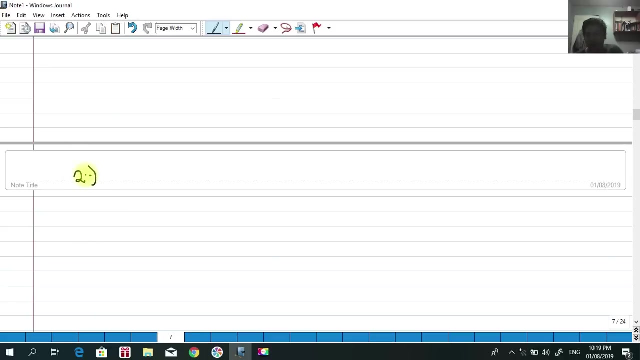 therefore, y of x, okay, y of x is equals to x raised to negative, 3 halves is a solution. okay, we have. only we only verify that. that given function is the solution for our differential equation. so let us try to verify some functions in a word: be so. 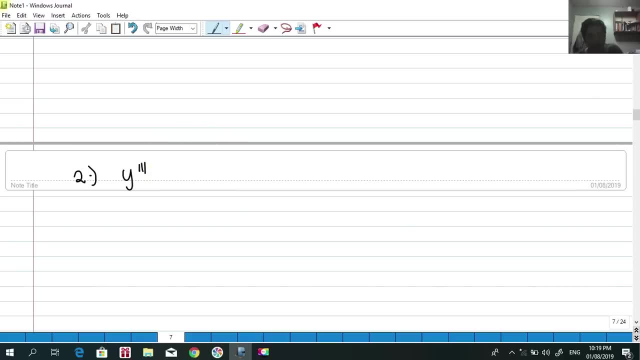 we have this: given: de is equals to 0 and we need to verify that this y is equals to e raised to negative 2. x is equal to y of minus 20 times x raised to aX raised to a solution to this dE. Again, we need to verify that this y is equal to e raised to negative 2x. 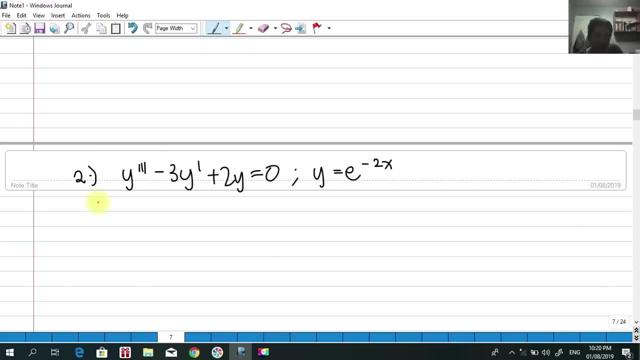 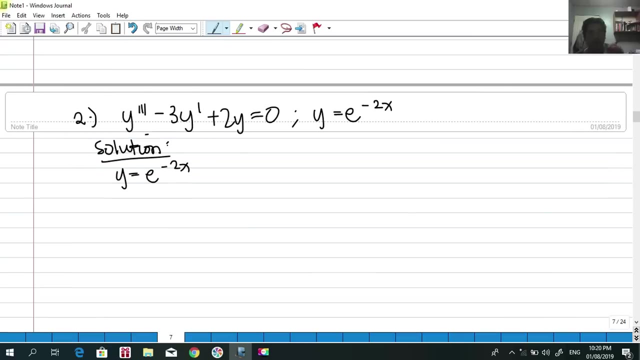 is a solution for this differential equation. Again, our solution would be: y is equal to e raised to negative 2x. We'll get the third derivative after the third derivative, because we have here the third derivative of y, y triple prime, So we have y prime that is negative. 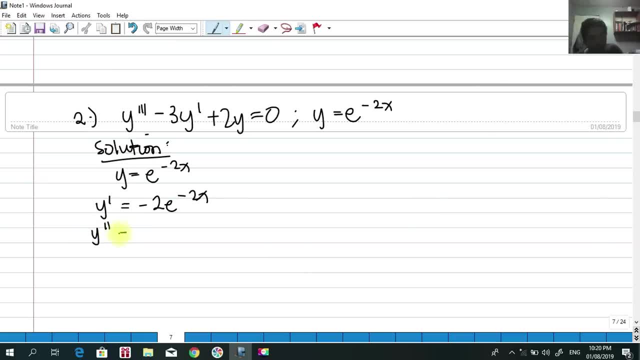 2 e raised to negative 2x. y double prime is 4 e raised to negative 2x. y triple prime is actually negative. 8 e raised to negative 2x. And what are we going to do? We simply substitute this y prime. 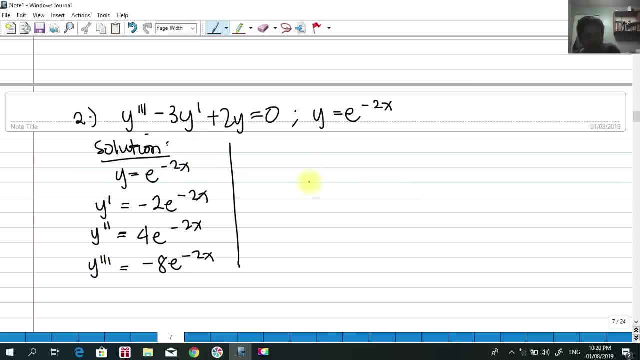 y triple prime or and y to this differential equation. So let's see. So our equation would now be: y negative 8. e raised to negative 2x minus 3, multiplied by y prime, negative 2 e raised to negative 2x- okay, plus 2. y which is e raised to negative 2x, is equal to 0.. So what will happen? 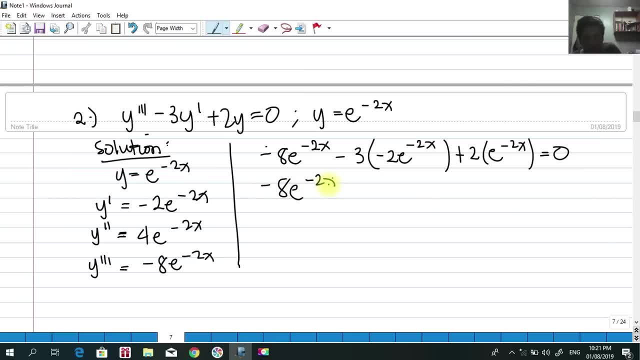 We have negative 8 e raised to negative 2x. Negative times negative, that would be positive 6 e raised to negative 2x. � and as you can see this would satisfy D equals 0. So this can be written as 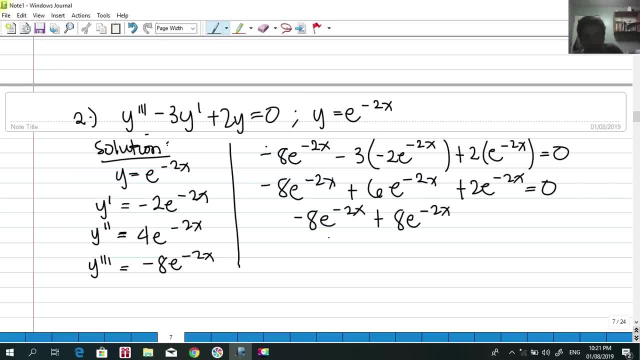 plus 8 e raise to negative 2x. So this is a negative 8. e raise to negative 2x. plus this, That should be equal to 0, so 0 is equal to 0, We verify that this Function is a solution Therefore. 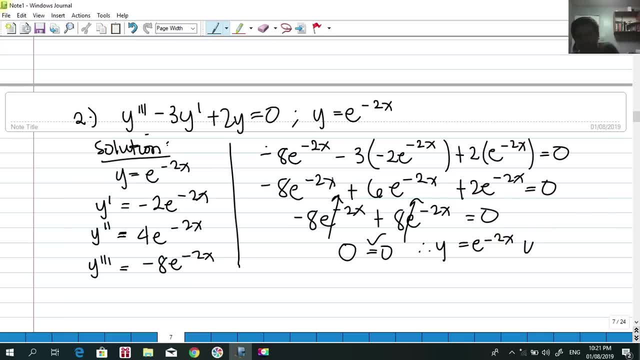 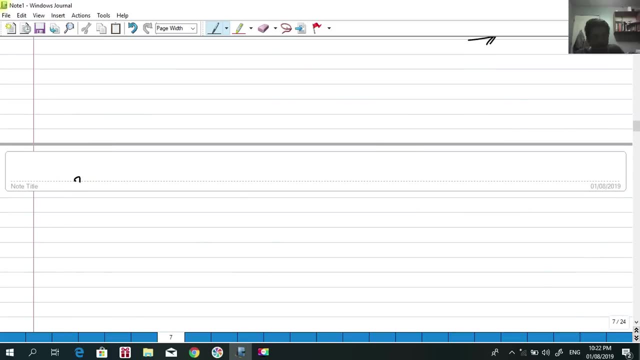 y is equal to e raised to negative. 2x is solution to our DE. okay, down to our third example, for us to be practiced here in verifying the solutions of DE. so for number three, verify again- this is the same question- that 3e raised to 2x. 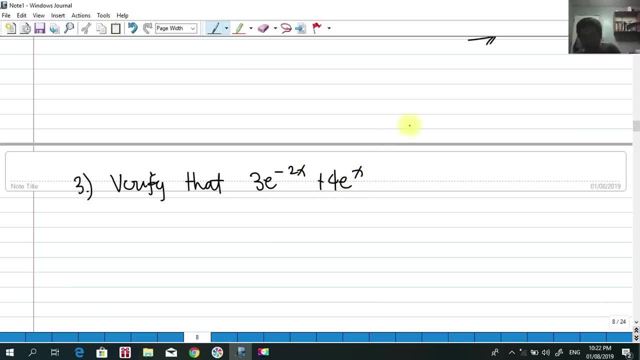 negative 2x plus 4e raised to x, is a solution of the differential equation. y triple prime minus 3y prime plus 2y. it's actually the same. okay, the. the differential equation is actually the same from the from the example above. so this is another solution, okay, just. 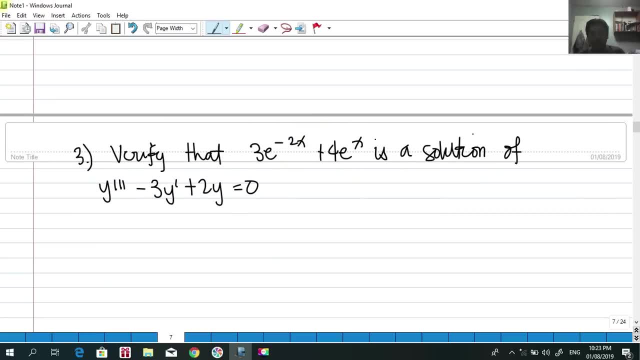 like in our polynomials, if we have two roots, then definitely that would still satisfy our equation. the same for differential equations. so let's try to solve this again. so for y we have 3e raised to negative, 2x plus 4e raised to x, so we need to get up to the third derivative. 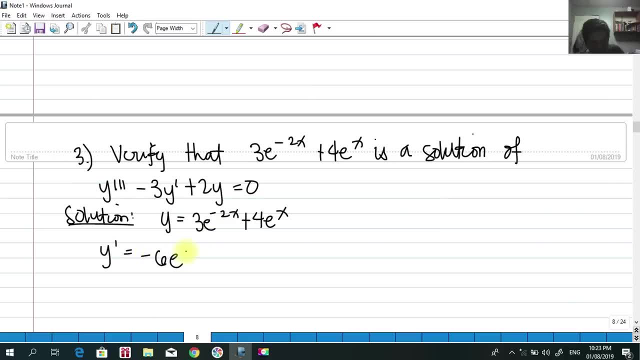 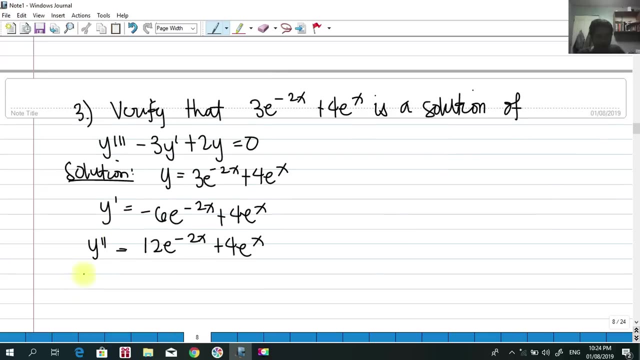 y prime is negative: 6e raised to negative. 2x plus 4e raised to x. y double prime would be 12e raised to negative. 2x plus 4e raised to x- okay and y, third derivative, would be negative. 24e raised to negative. 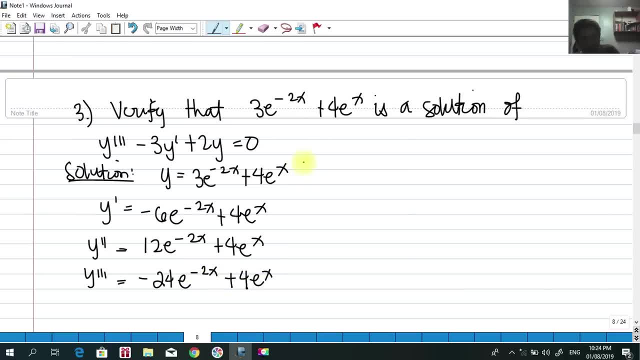 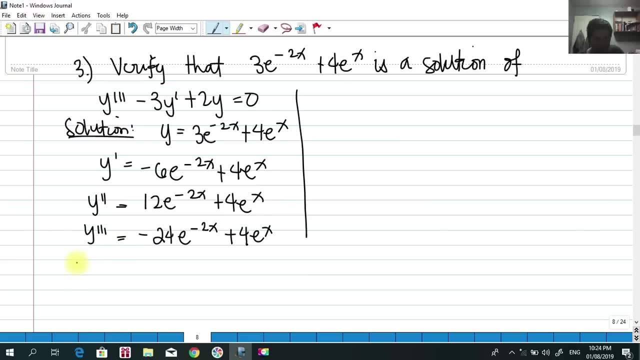 2x plus 4e raised to x. okay, again, we substitute it to the original differential equation. so now we have- oops, let me just rewrite this on the lower side so that we'll have enough space. so we have y triple prime that is negative 24e. 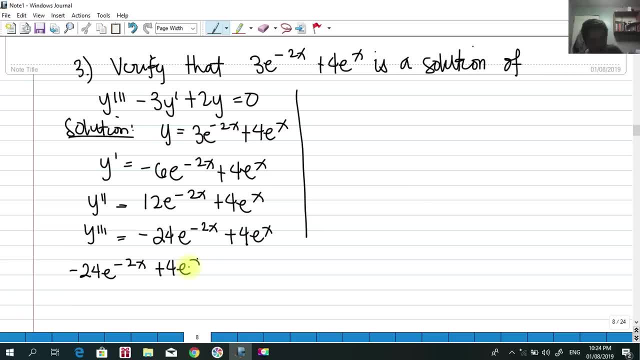 raised to negative, 2x plus 4e raised to x, that is our y triple prime minus 3 times the y prime, which is negative. 6e raised to negative: 2x plus 4ex plus 2 multiplied by the y, which is simply 3e raised to negative 2x plus 4e raised to x, is: 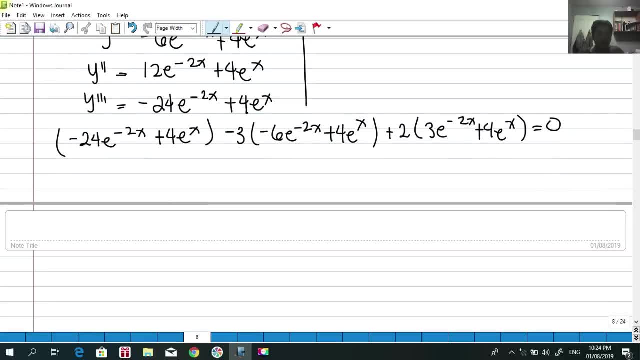 equals to zero. simplifying. we have negative 24e raised to negative 2x plus 4e raised to x. distributing this, so we have plus 18e raised to negative 2x minus 12e e raised to x. okay, minus 12. e raised to x plus 6 e raised to negative 2 x plus 8 e raised to x. 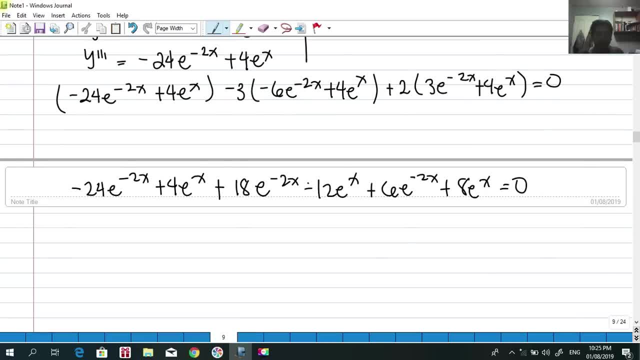 is equal to 0 and again, if we combine like terms, so we have negative 24 e raised to negative 2 x plus 18 e raised to negative 2 x plus 6 e raised to negative 2 x. so, as you can see, 18 plus 6 is 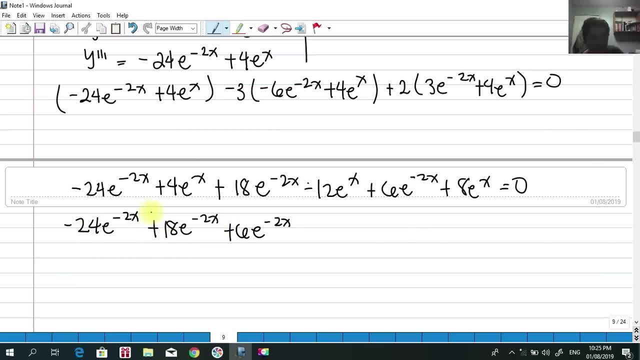 24. we need to minus that into this, so definitely that would cancel. so plus 4 e raised to x, 4 e raised to x and uh, minus 12 e raised to x. plus 8 e raised to x is equal to 0. so if we are going to simplify these equations, so we have negative 24 e raised to negative 2 x. 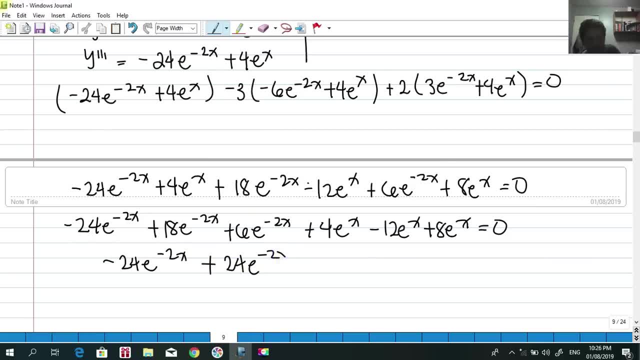 18 plus 6, that is 24 e raised to negative 2: x. you can see these two would cancel. okay. and 4 e raised to x plus 8 is simply 12 e raised to x minus 12 e raised to x equals to 0. definitely. 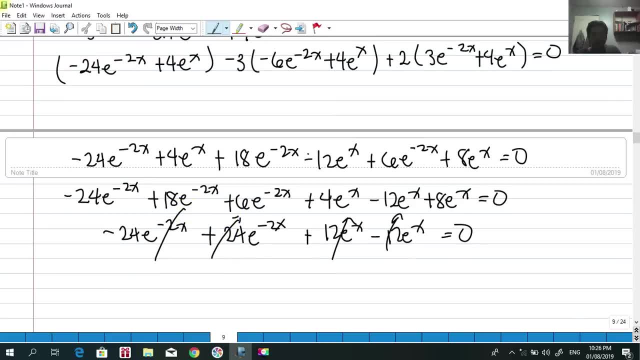 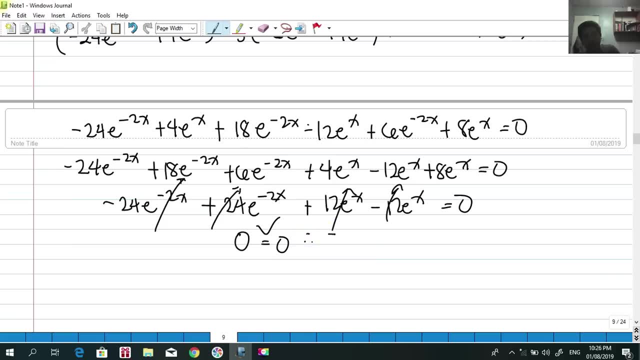 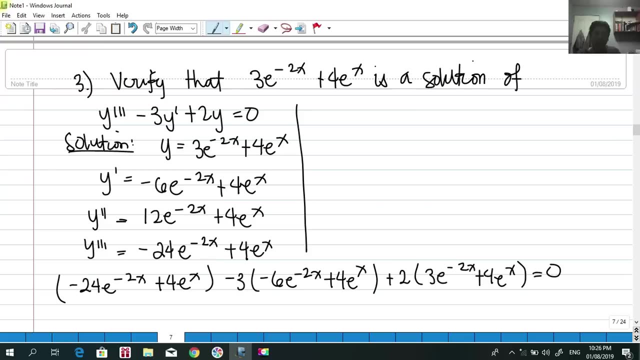 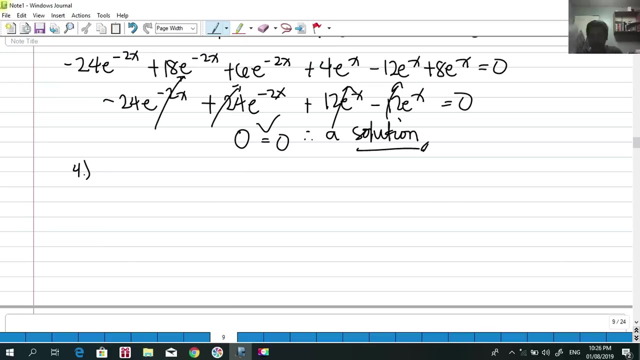 this given equation or function is a solution of our b, therefore a solution. okay, so the given is actually a solution of our differential equation. and down to our last example, for our last example, this is the easiest one. okay, so we need to verify, verify that the solution of the